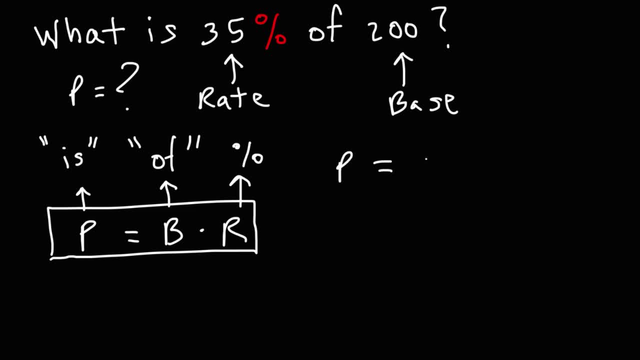 So we want to calculate P in this problem. The base is 200 and the percentage is 35%. That's the rate I mean. let me not confuse that with P and R. R is 35%, So what is 35% as a decimal? 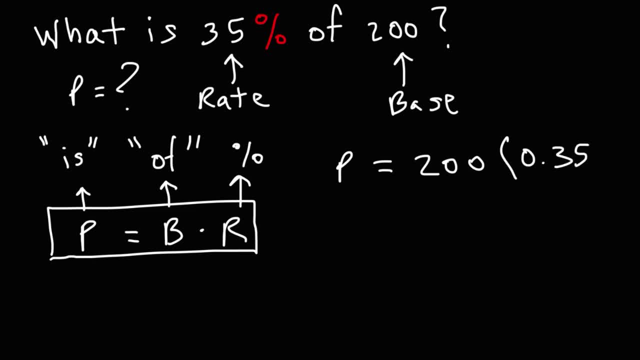 35% as a decimal is 0.35. So all we need to do is multiply 200 by 0.35. And you'll get 70.. By the way, to convert a percentage into a decimal, simply move the decimal point two units to the left. 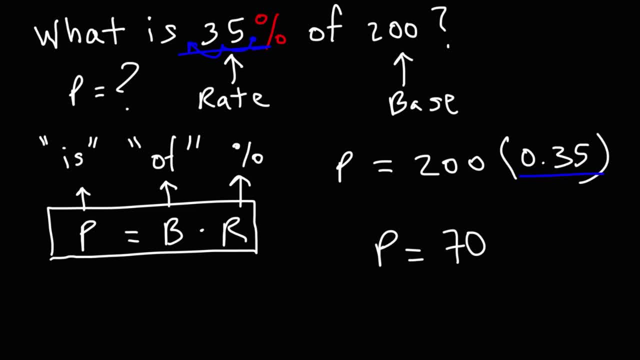 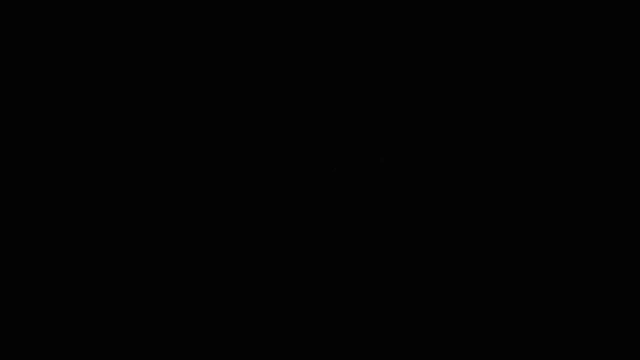 or you could take 35 and divide it by 100. Both ways will give you 0.35.. But for this problem, 70 is the answer. So 70 is 35% of 200.. Now, for the sake of practice, let's go ahead and try another example. 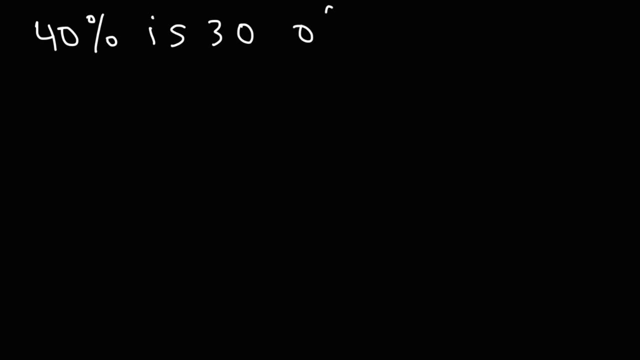 40% is 30? of what Number? Feel free to pause the video and try this example problem. So let's use the formula again. Percentage is equal to the base times the rate, So let's identify what we have: 40%, even though it has the percentage symbol in front of it. 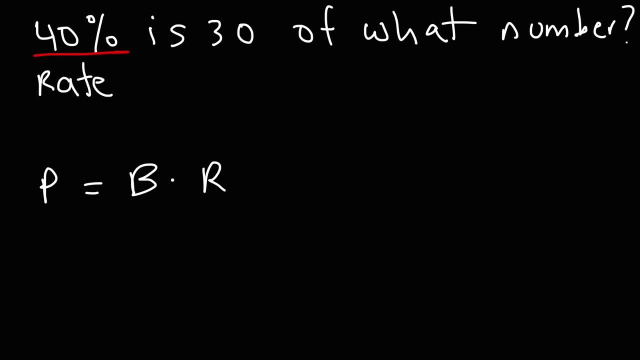 That is the rate. Now, what about 30 is 30?? What does that tell us? The number that is associated with the word is is the percentage, So that's P. And then of what number? that's what we're looking for. 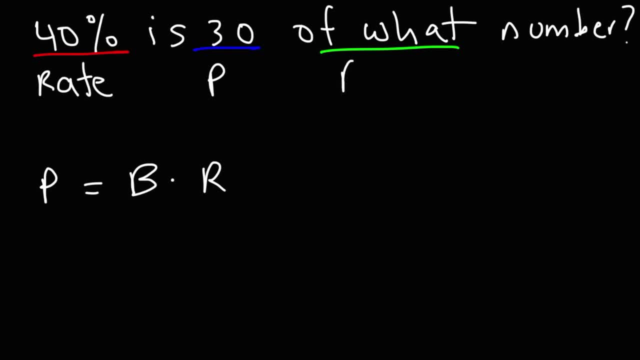 So in this problem we're looking for the base B. So that's what we need to calculate in the equation. Now let's plug in what we know: P is 30.. We don't know the value of the base And we know R: the rate is 40%. 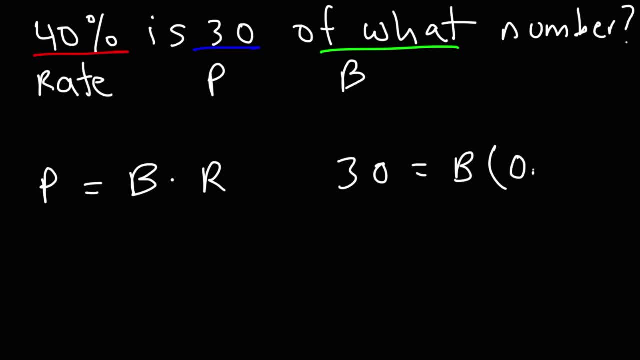 So we know that the rate is 40%. So 40 divided by 100 is 0.40.. So now we'll need to do a little math here. How can we calculate B, the base, In order to get B by itself on the right side of the equation? 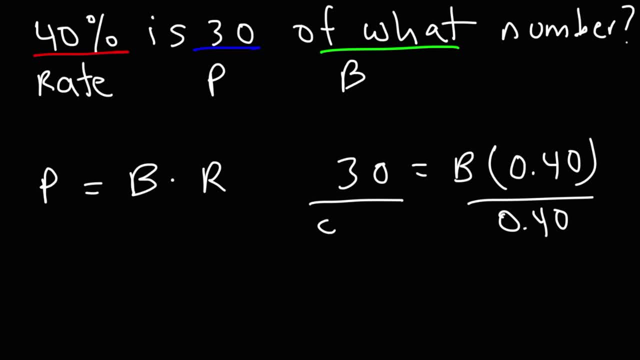 we need to divide both sides by 0.40.. 0.40 divided by itself is 1.. So those two numbers will cancel. So on the left we have 30 divided by 0.40.. And that will give. 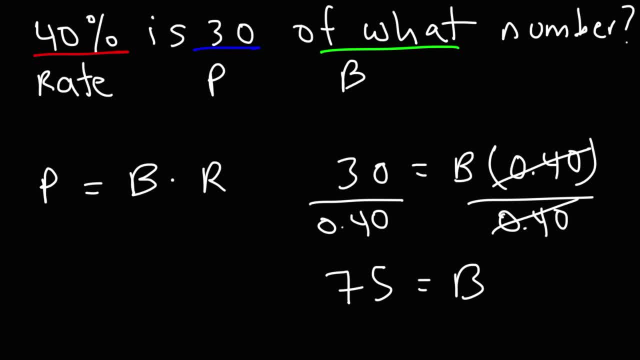 That will give us 75.. And so that is the base, That is the answer that we're looking for. So we can say that 40% is 30 of 75.. So that's how we can complete the sentence. Now let's move on to our next example. 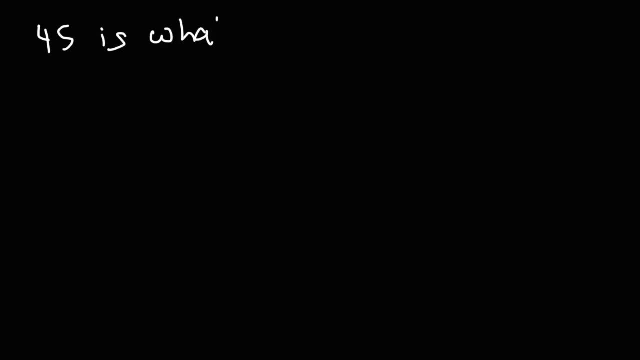 45 is what percent of 70?? Go ahead and work on that example. So let's use the same formula. P is equal to B times R. So what's P, what's B and what's R in this problem? So P is associated with the word is. 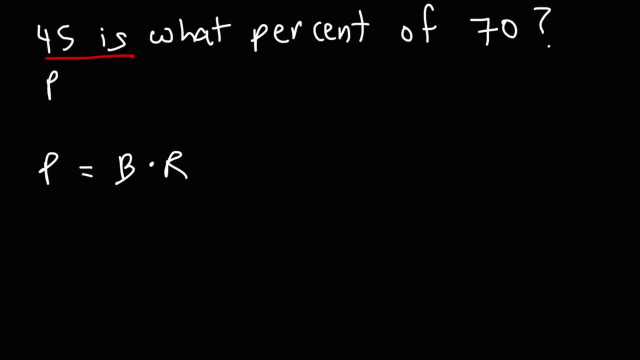 45 is, So 45 is going to be P. Of is associated with the base, So 70 is the base. The percentage in this formula is associated with R, the rate. So in this example we want to calculate the value of R. 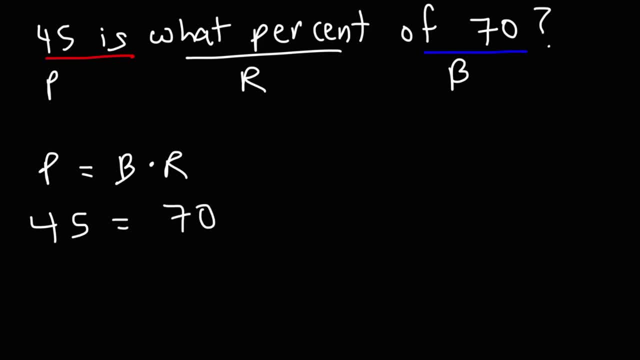 So P is 45.. B is 70. And now we need to get R by itself. To do that, let's divide both sides by 70. So R is going to be 45 divided by 70. And we're going to get a decimal. 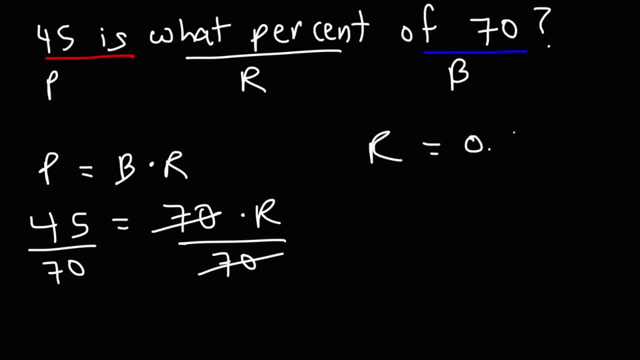 So you should get 0.6428571.. And we're going to round it. We're going to say: this is approximately 0.643.. Now that's as a decimal. We need to convert that into a percentage. To do that, you can multiply 0.643 by 100 or move the decimal two units to the right. 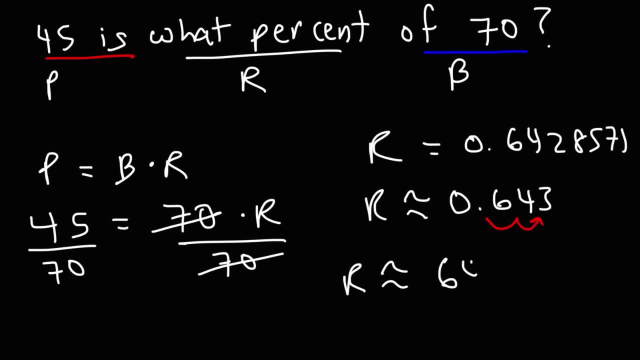 So R is approximately 64.. 0.3%. So we can say that 45 is approximately 64.3% of 70.. So that is our answer. So that's it for this video. So now you know how to solve these percentage-based rate problems.